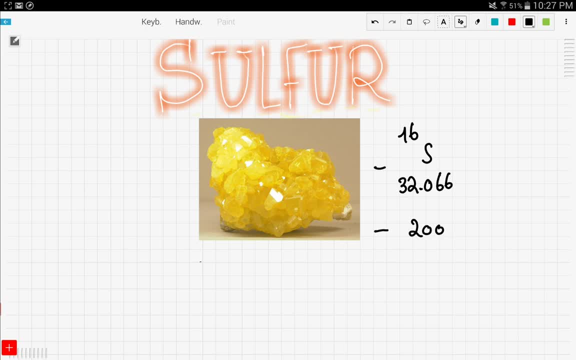 Sulfur was first discovered by the Chinese people in around 2000 BCE- so it's a while back- And it was officially discovered by a French chemist called I know- I didn't pronounce it perfectly because I'm not French educated, but if you're interested in him, just google his name. 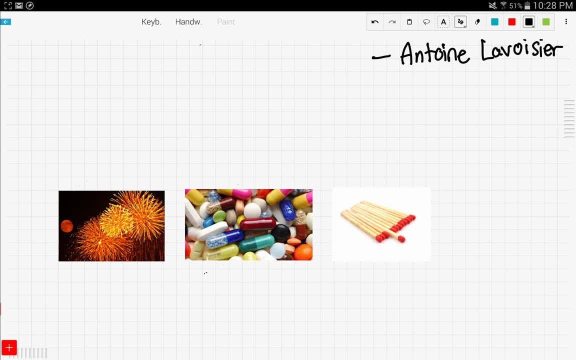 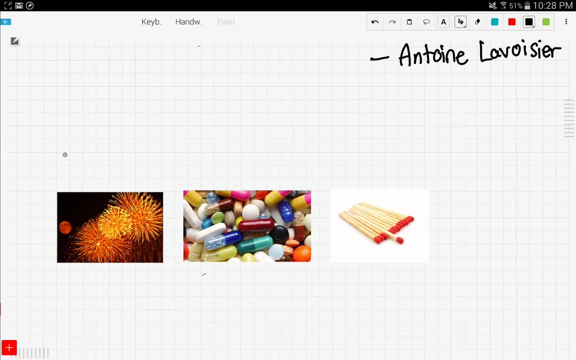 Okay, so let's take a look at these three different pictures. Well, I don't know if you guys can guess what's the common thing between them, but let's take a look. Okay, the first picture right here is a picture of fireworks. 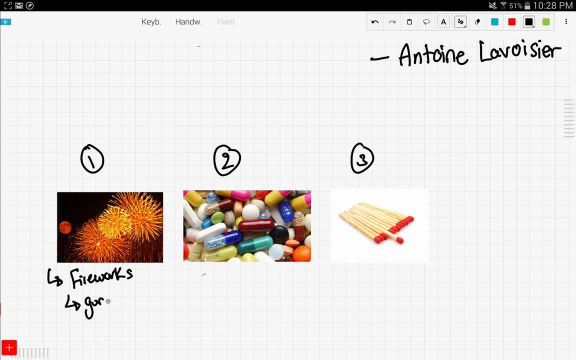 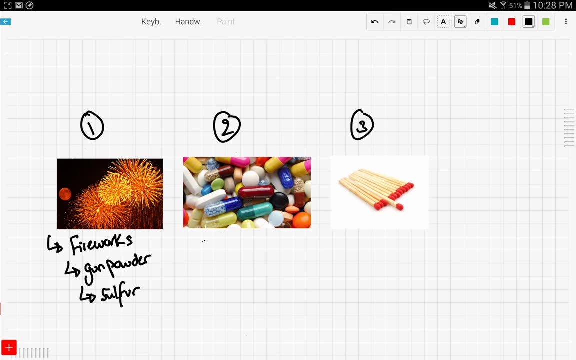 And And fireworks contain gunpowder, And gunpowder contains sulfur, And sulfur is responsible for this bright red color, Although sulfur is yellow colored in nature, but when it ignites in air it causes this red color. Okay, let's take a look at the second picture, which is a picture of medicine. 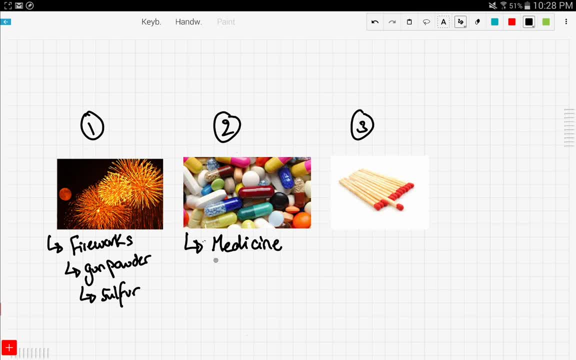 Well, nobody likes taking meds, but if you're experienced, you should know that it's a very good thing. Also, if you're experiencing any acne problems, your acne meds would contain sulfur, as it aids in the process of healing your acne. 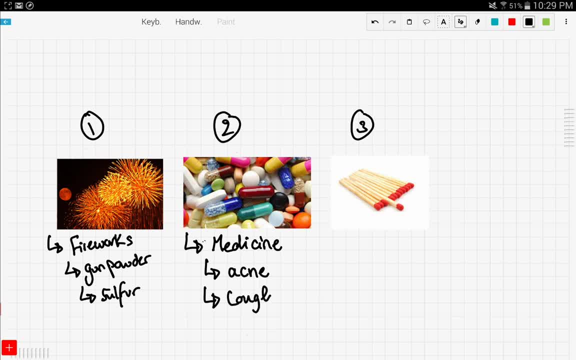 Also, if you're experiencing any coughing or bronchitis, God forbid that, but your meds would contain sulfur. Okay, the third picture is a picture of some matches, and matches also contain gunpowder And, as we learned, gunpowder contains sulfur. 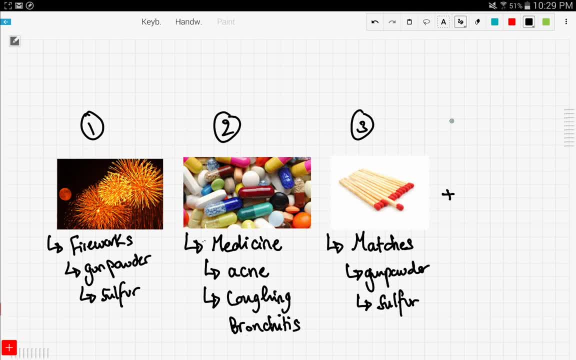 Okay, in addition to all of these, you know those lovely trees and plants and flowers. well, farmers put some fertilizers in the soil in order to aid the growing process of the plants. Lizers, okay, And fertilizers contain sulfur. 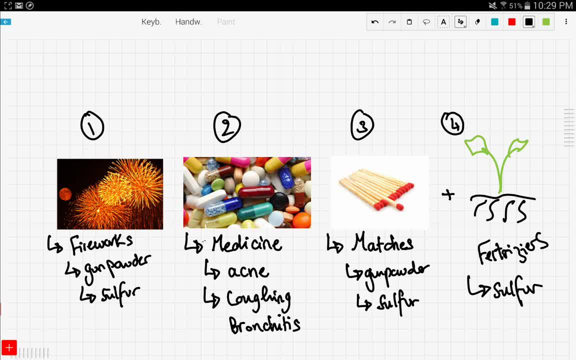 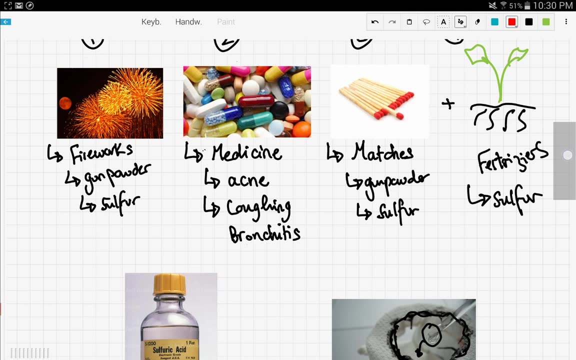 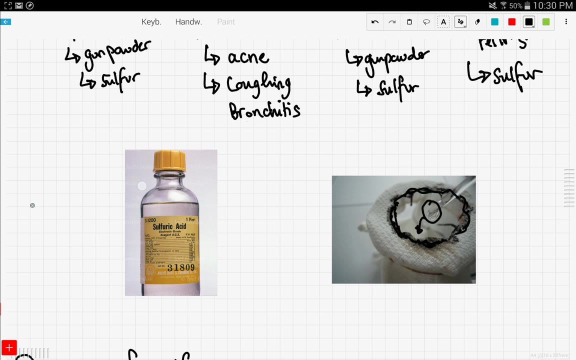 Because sulfur has an antifungus property that kills fungus in the soil. So these are the different uses of sulfur in everyday life. Okay, Now let's take a look at some of the chemical uses of sulfur. Well, one of the main chemical uses is production of sulfuric acid, which has the formula of H2SO4.. 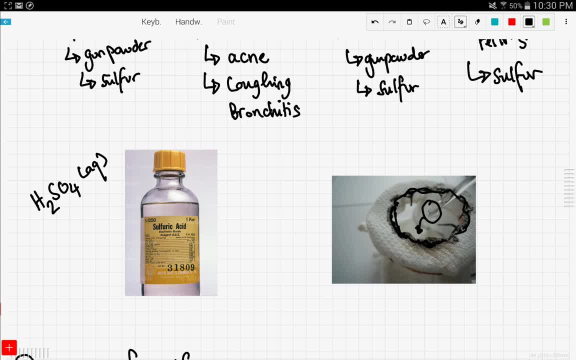 Okay, And sulfuric acid is very harmful to the skin, skin and clothes. it can cause burning and i'm sure your lab instructor told you not to get it anywhere on your skin or your hands because it can cause burning. let's take a look at this picture. 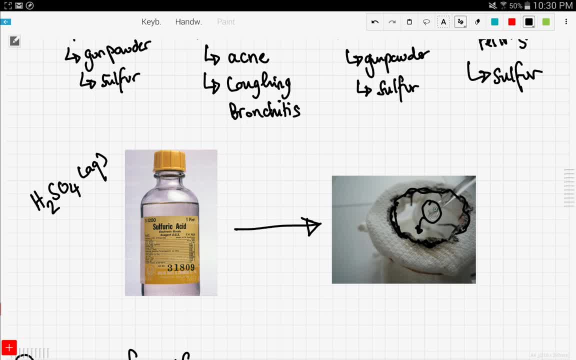 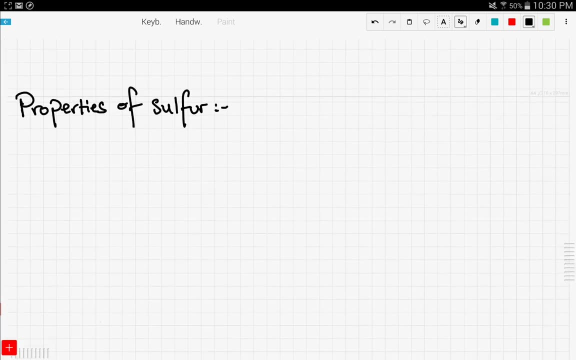 right here it's a picture of someone dropping some sulfuric acid on a cotton cloth and it causes burning. so you can see the harmful effect of sulfuric acid. now let's move on to some of the chemical properties of sulfur. well, the first property we're going to look at is that sulfur. 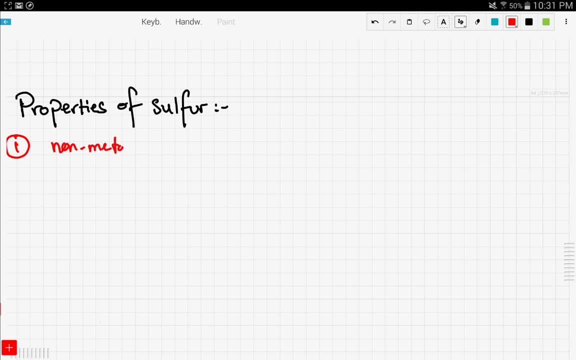 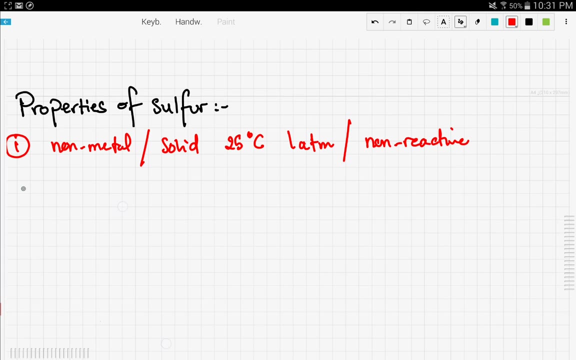 is a non-metal and it's found a solid in normal conditions, which is 25 degrees celsius and one atmospheric pressure. it's also non-reactive at these conditions. okay, but sulfur can react under other conditions and it's react with both metals and nonmetals- with both metals and nonmetals, let's. 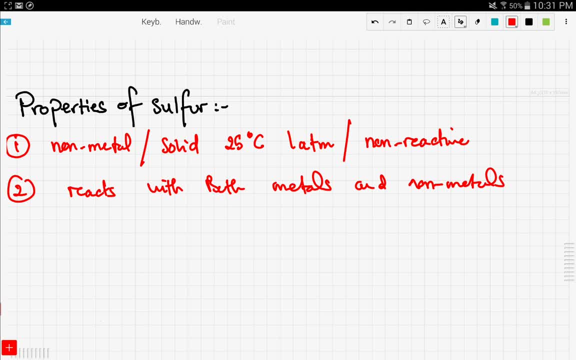 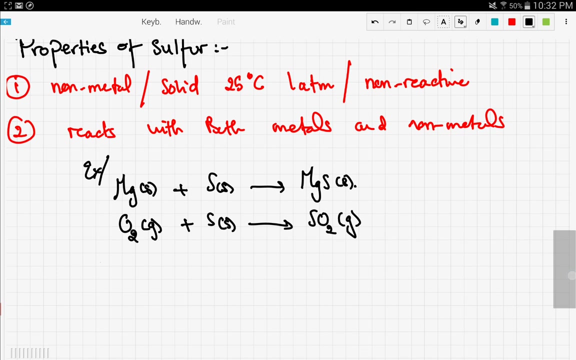 take an example. well, magnesium solid, which is a group two metal, reacts with sulfur solid to give magnesium sulfide. also, sulfur reacts with oxygen gas to give us sulfur dioxide, and sulfur dioxide is the gas responsible for acid rain. and now we're going to talk about acid rain more, because it's very